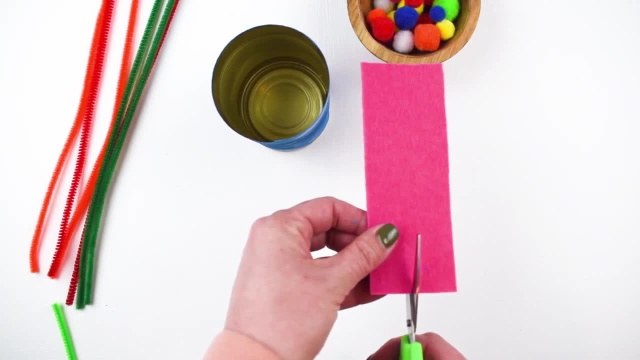 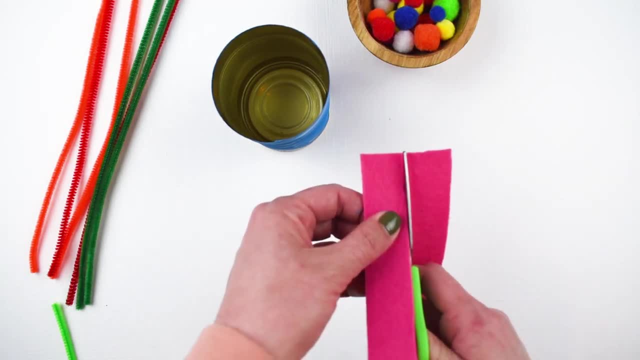 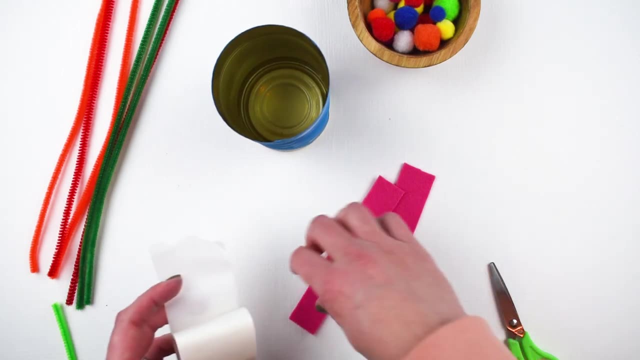 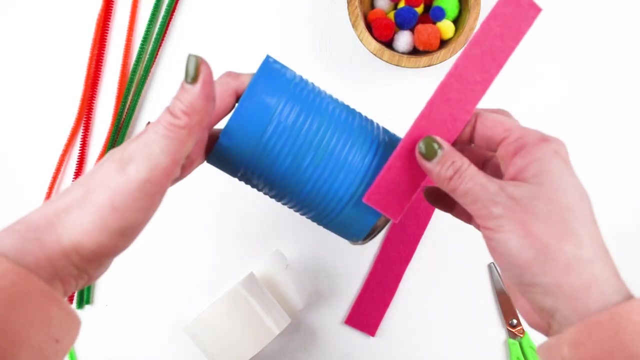 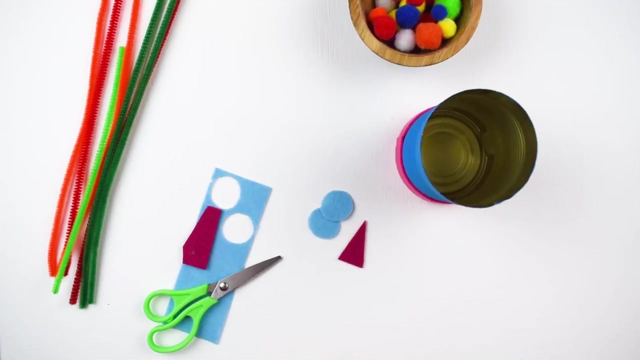 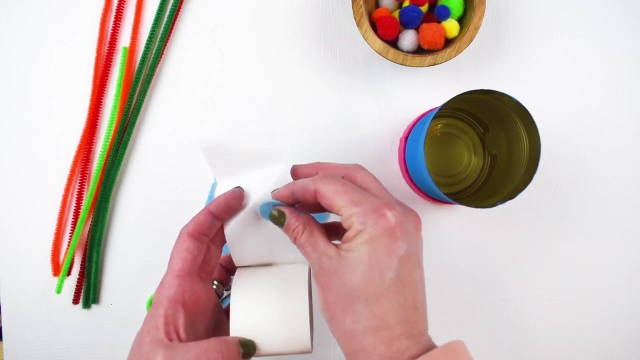 And, using glue dots, attach it to the bottom of your planter. Use scissors to trim off any extra felt. Cut two quarter sized circles out of another color felt strip and a triangle for a nose. Add a single glue dot to the back of each felt shape and attach to the front of your 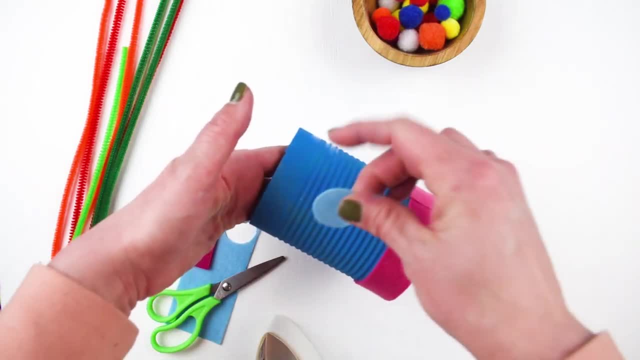 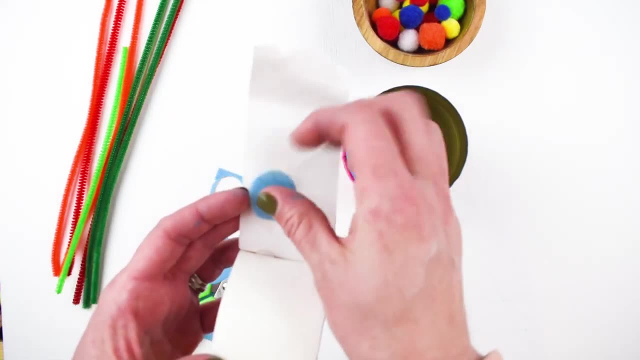 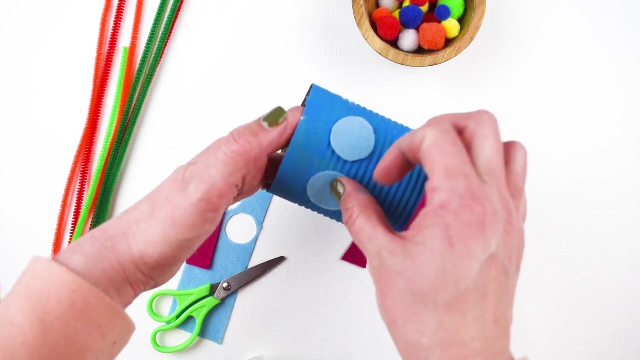 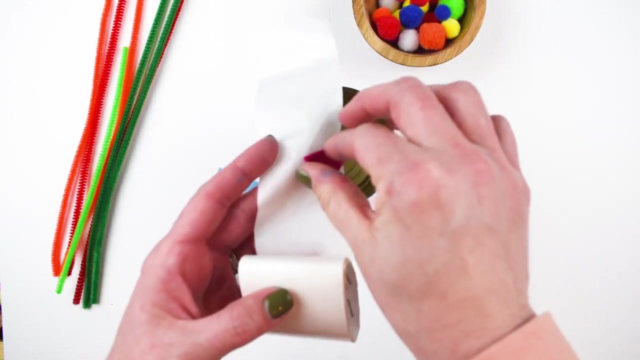 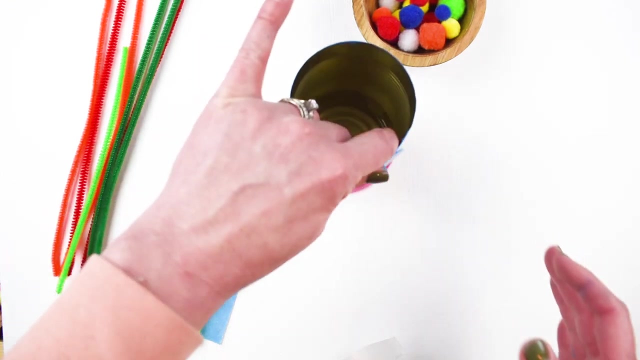 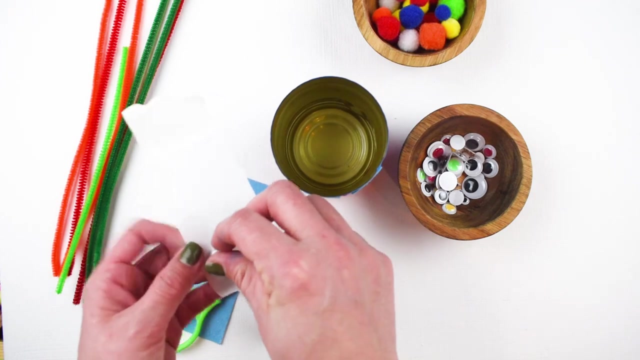 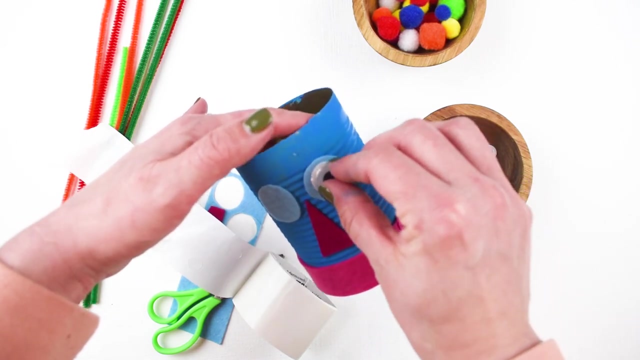 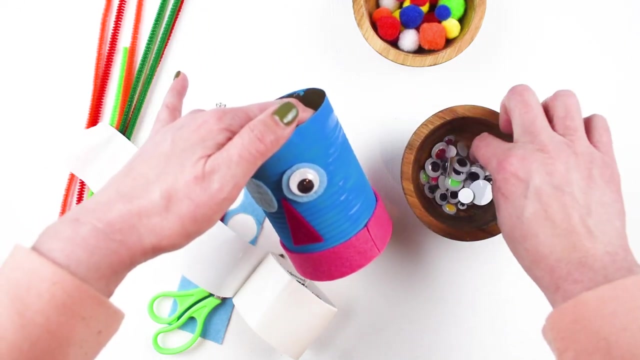 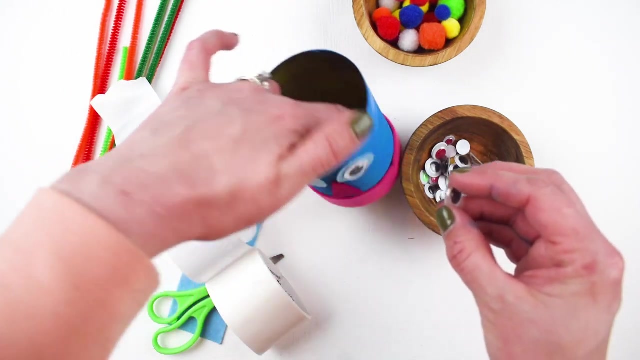 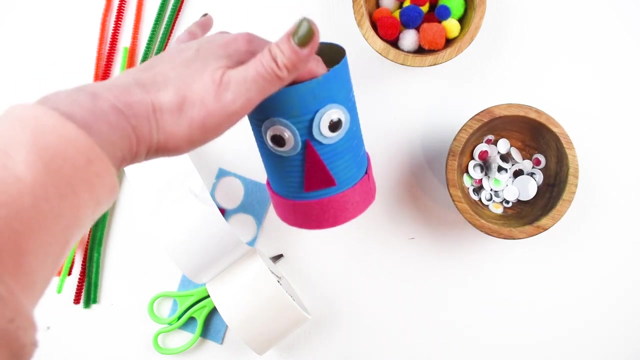 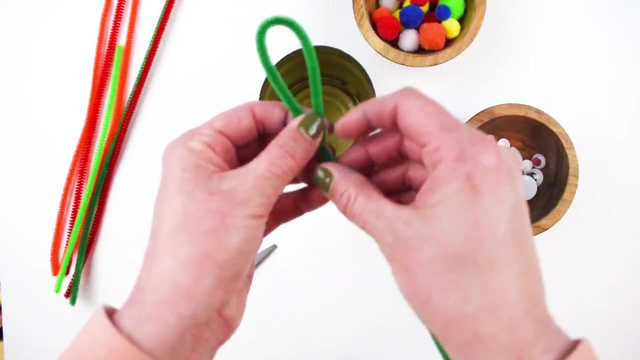 planter to create a face structure. Attach googly eyes in the center of your felt circles to complete a funny face for your planter. Continue adding some fun details to your planter. I chose to create a bow tie by bending a fuzzy stick into a bow shape and gluing it to the bottom of the planter. 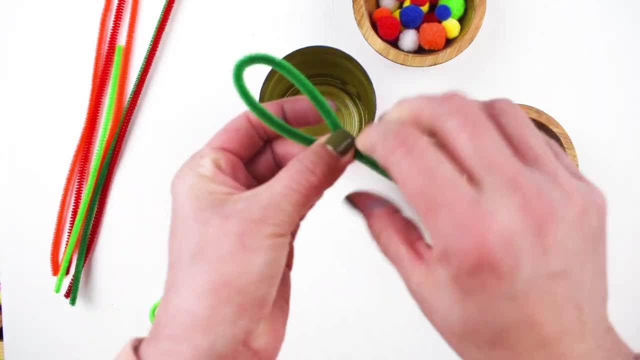 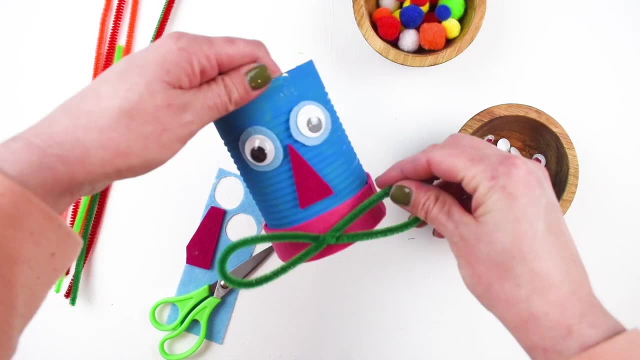 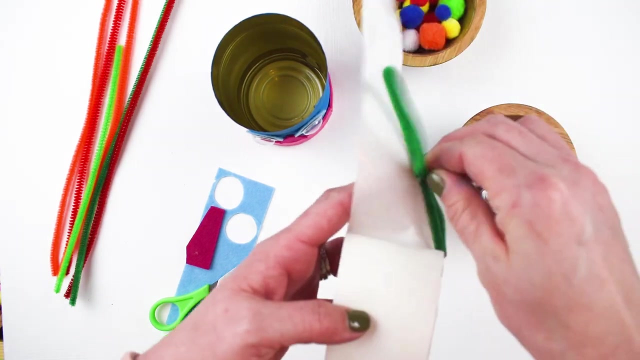 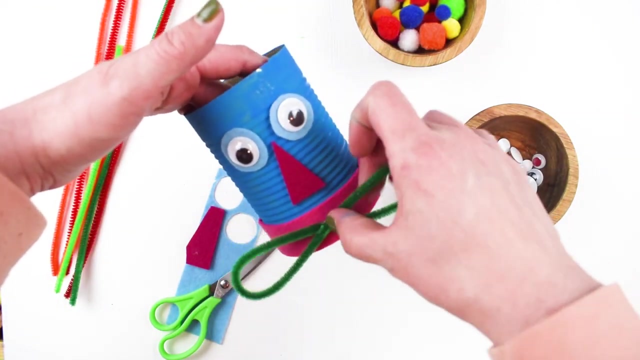 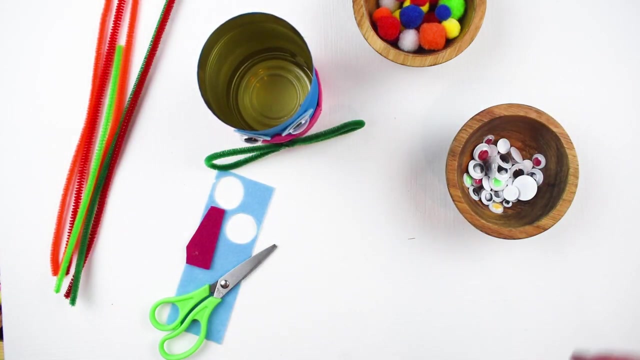 Add a pom pom in the center to complete the style. Add, on top of everything, a lady band. Use a plastic board toumbled into a bow tie. Loop around your entrepreneurs circle to create a bow tie. Make sure that you have straight lines. 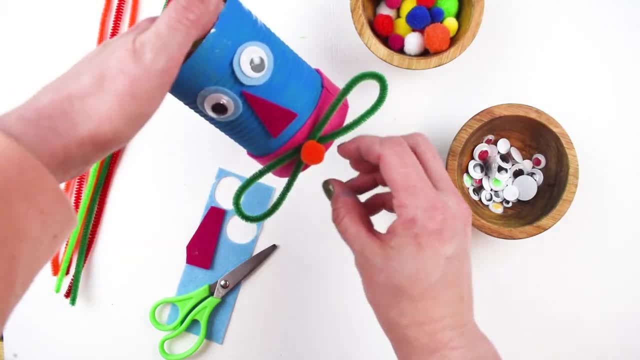 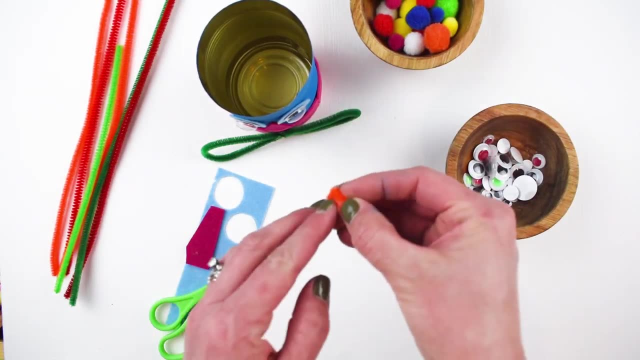 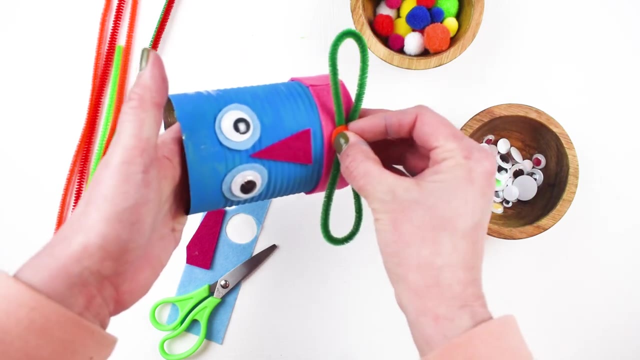 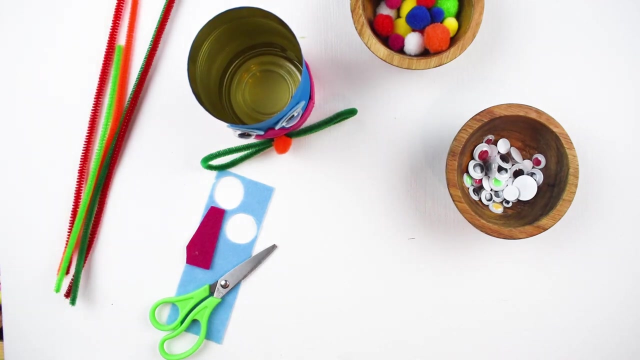 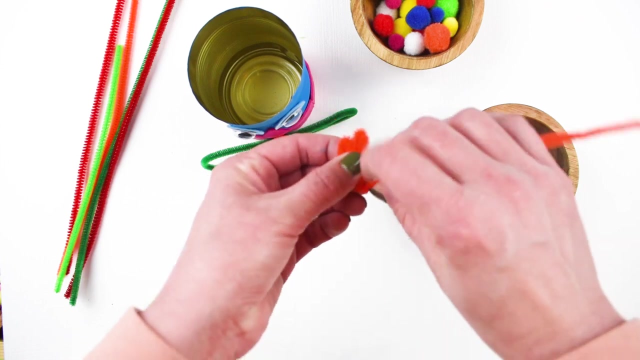 This will slow the bliss of your kita technique and also help in creating more consistency. Add a shell made of slabs. Add loweräter to a piece of hollow glass or a bambooства. Next fold two fuzzy sticks into a zigzag line by folding one inch increments up and back down to create the pattern. 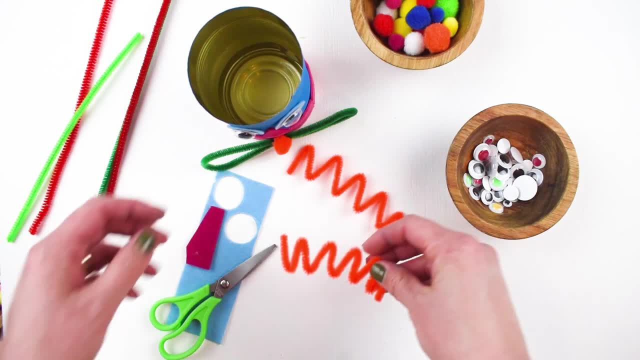 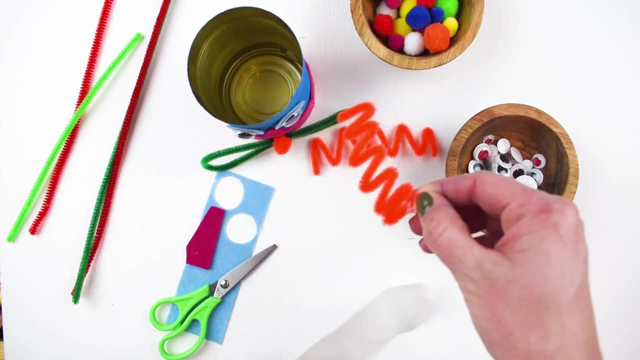 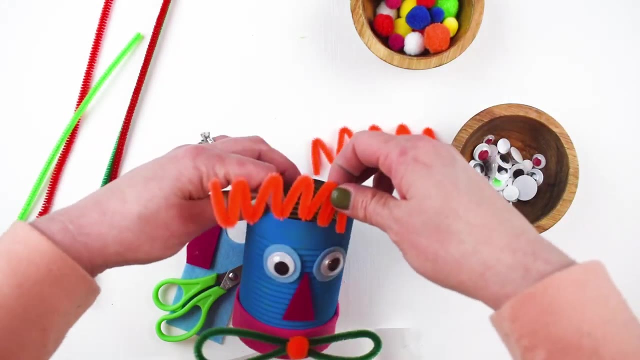 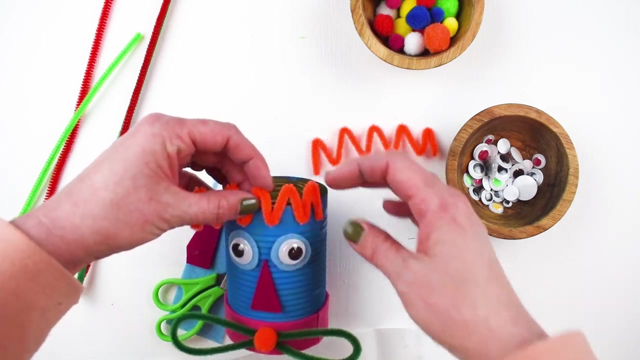 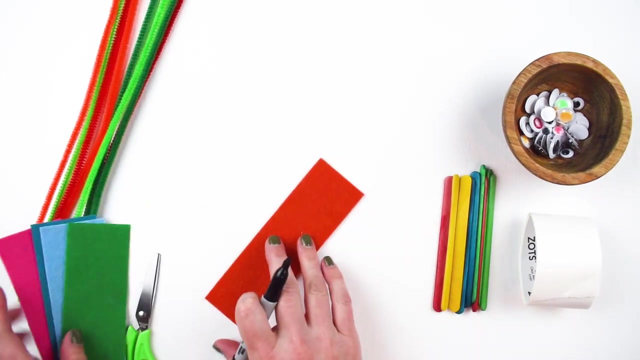 Add a glue dot to every other folded portion and attach to the top of your planter to resemble a crown or hair. Keep adding more details and get creative. When you're finished, it's time to move on to creating our garden markers. The first garden marker we're going to create is a carrot. 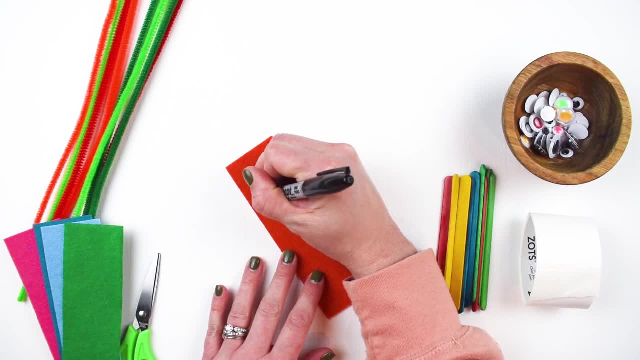 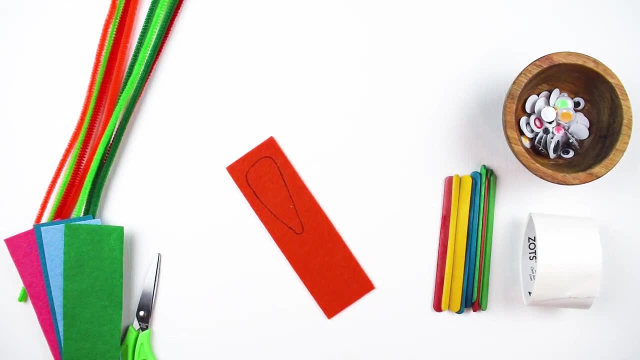 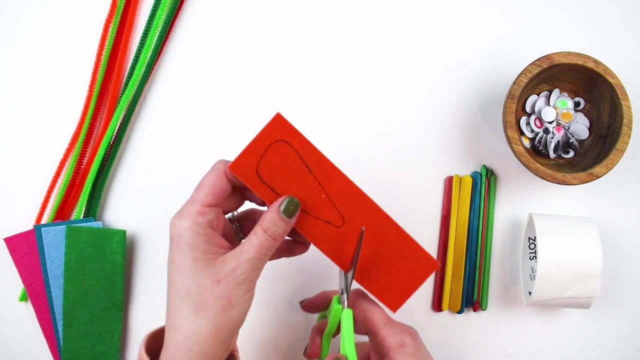 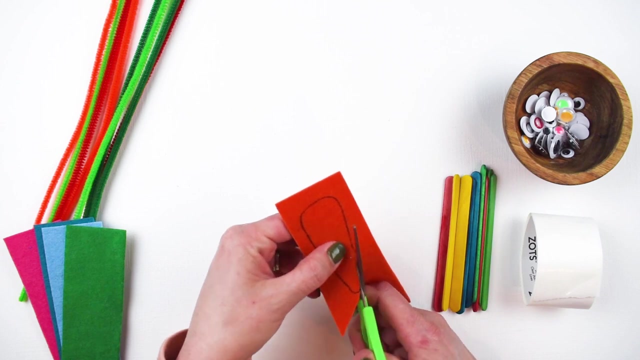 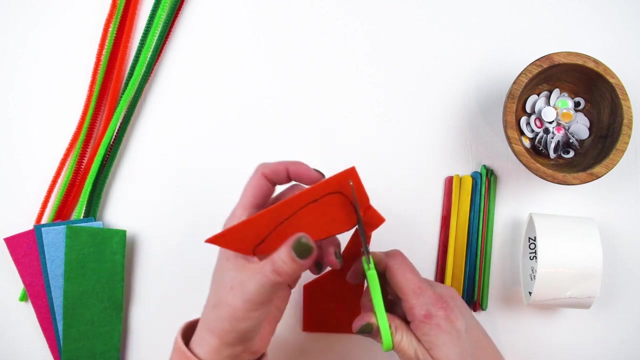 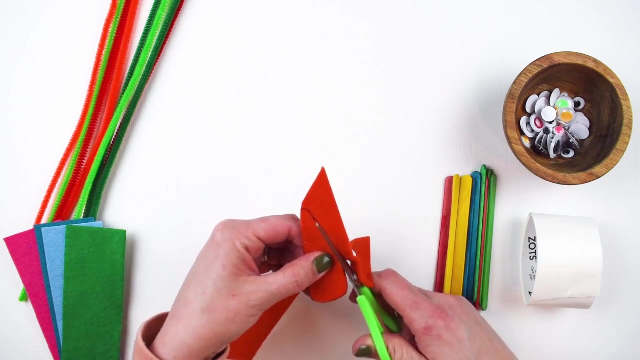 Using an orange felt strip and marker, draw a rounded triangle shape to look like a carrot and cut along the marker line. We have made our paper runner. jetzt Прошу不要 забTY�� ваше внимание. and see a few scissors and shovels. 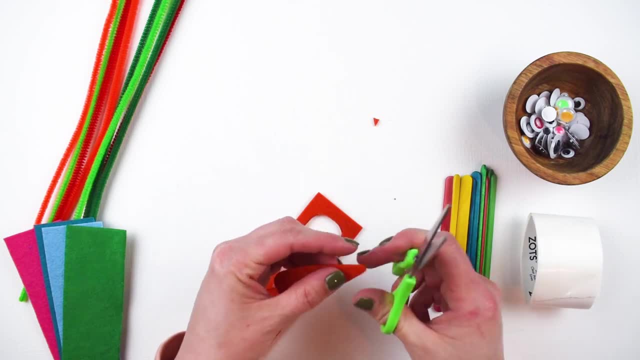 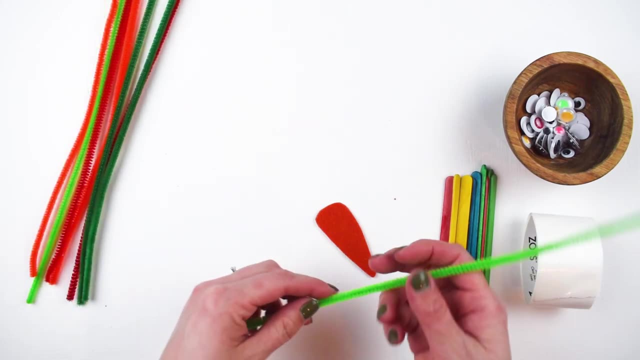 Then tap the pencil at the start needle and thread those chapters toそして wrap it to the basket. The same process with the cut turns over and mark the spot. Have fun, Bye, Bye, Bye. Cut a portion of a green fuzzy stick and bend it into a tight zigzag, bending it up and 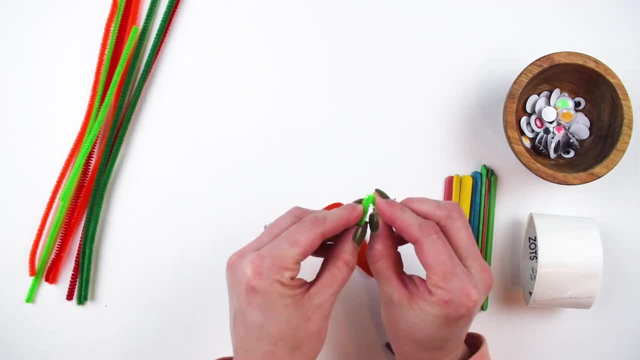 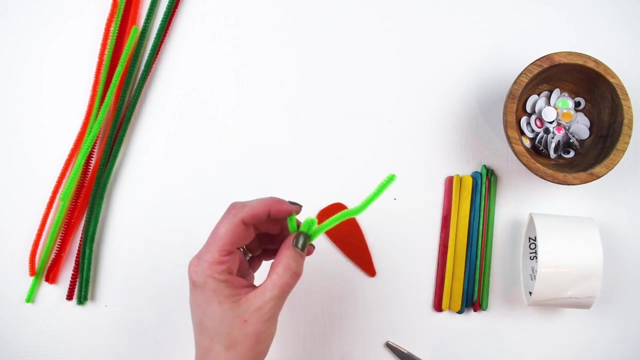 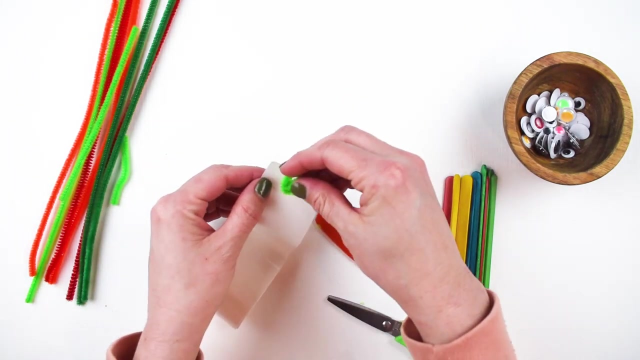 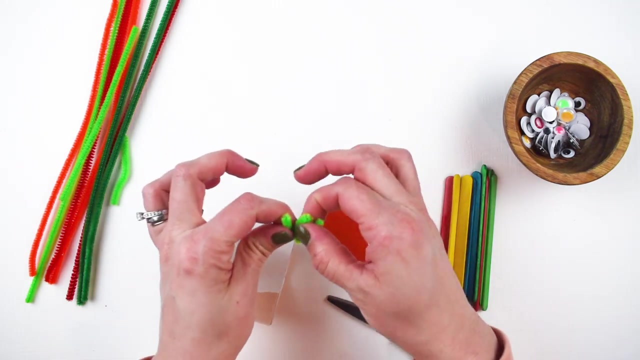 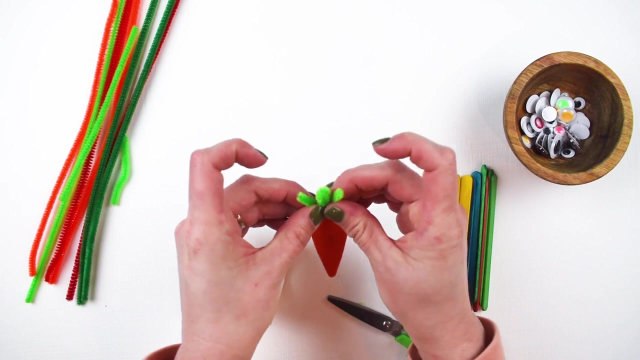 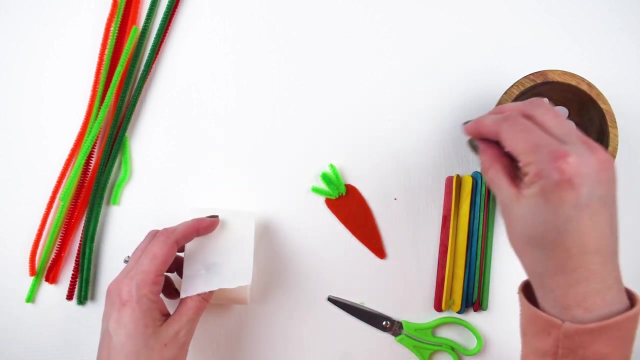 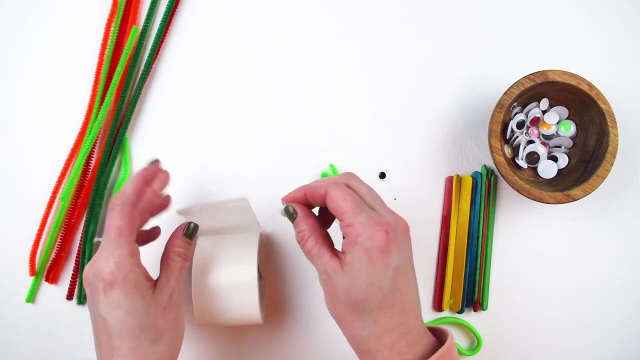 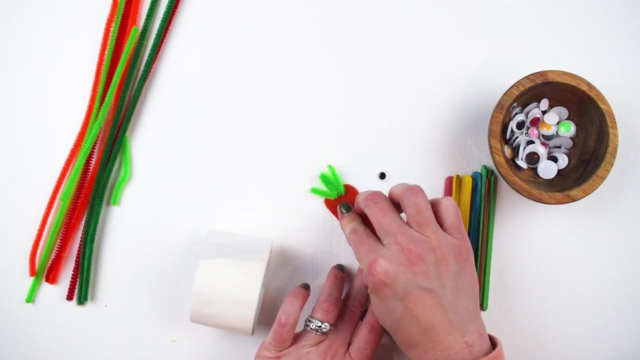 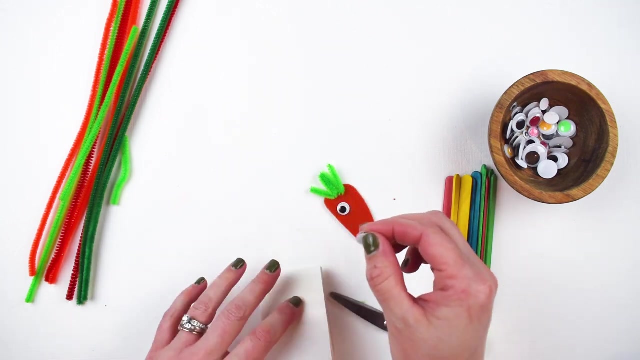 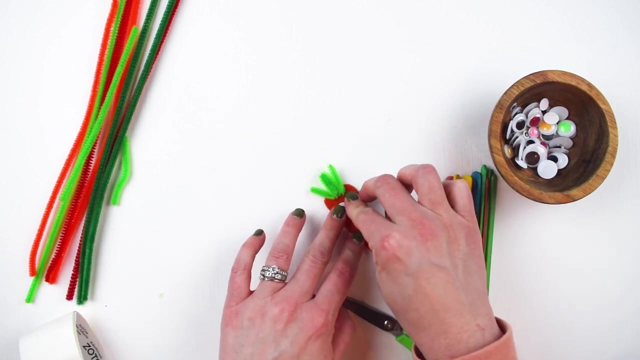 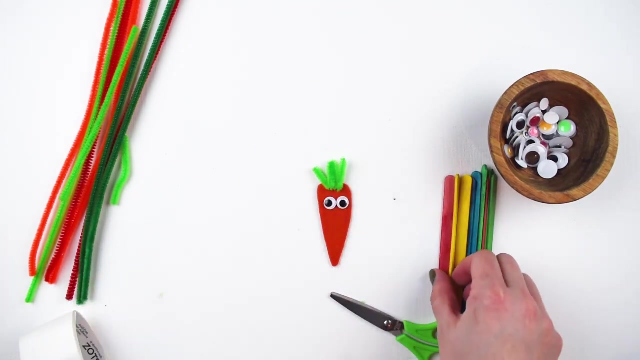 back down three times to create a carrot top. Attach it to the top of the felt carrot with a glue dot. Add two small googly eyes with glue dots to the top of your carrot to give it some personality. Lastly, turn the carrot over and attach a. 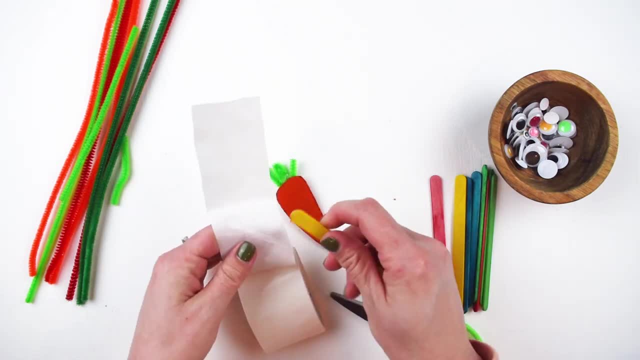 wooden cross to the top of your carrot. Attach a wooden cross to the top of your carrot to give it some personality. Attach a wooden cross to the top of your carrot to give it some personality. Use two to three glue dots at the top of the craft stick and press it against the back of your carrot. 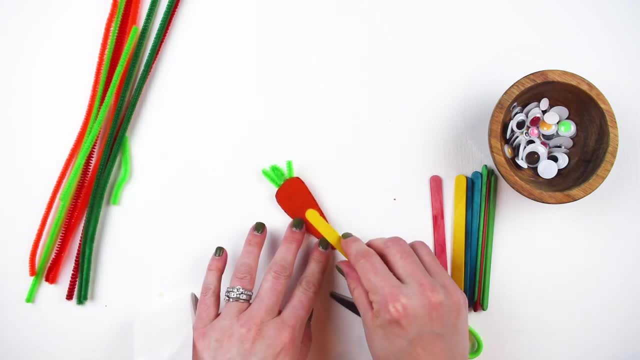 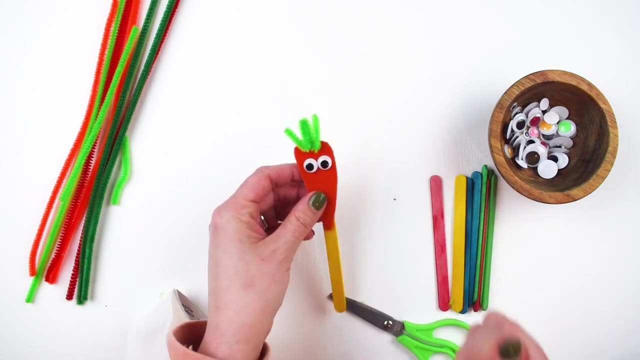 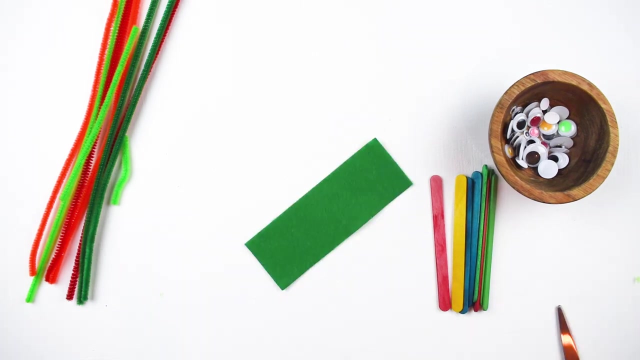 Your garden marker is ready to stick in your new veggie garden. Now you can use the same materials to create a marker for every type of veggie you plant in your new recycled can garden. Let's make one more option to give you a little extra inspiration. 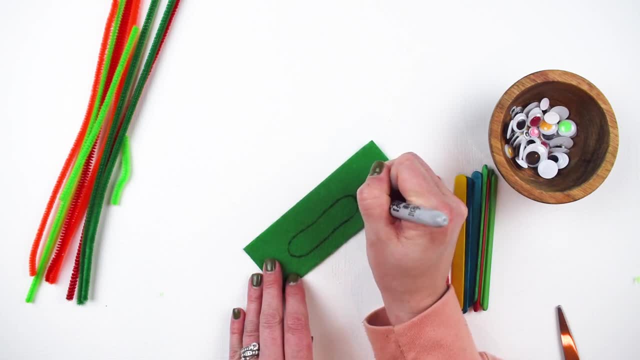 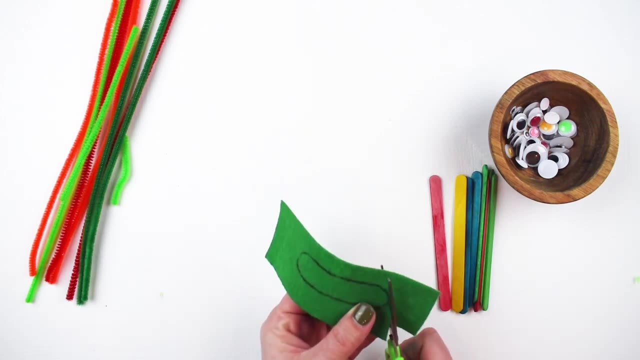 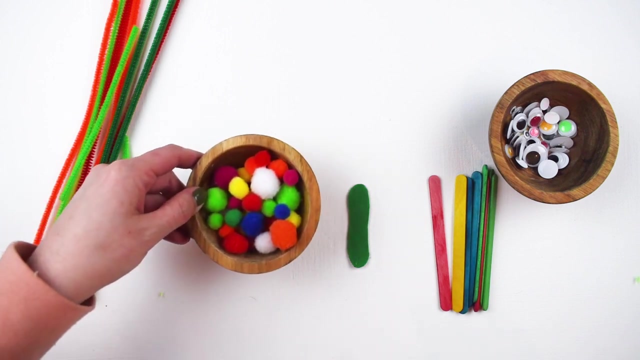 For this next garden marker we will make a pea pod. Draw a long oval shape on a green felt strip and cut it out. So, using small pom-poms, glue three palms in the center of the green oval you just cut out. These will look like little peas in a pod. 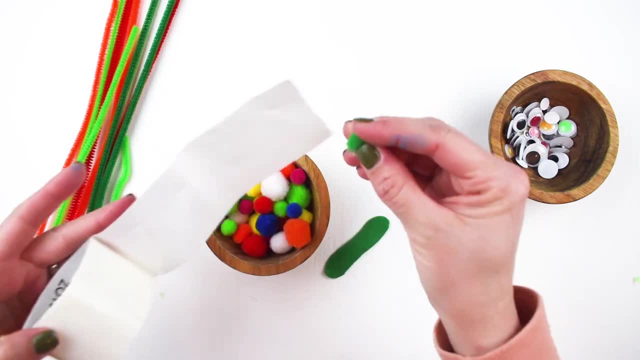 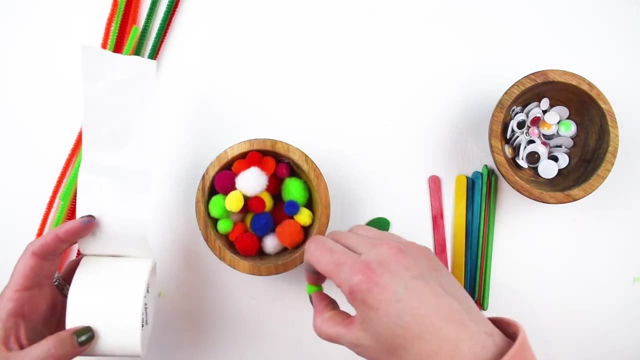 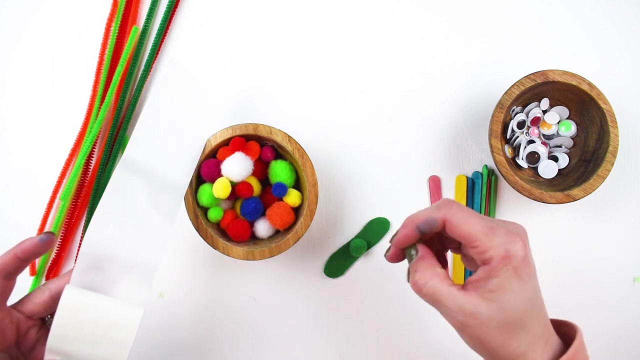 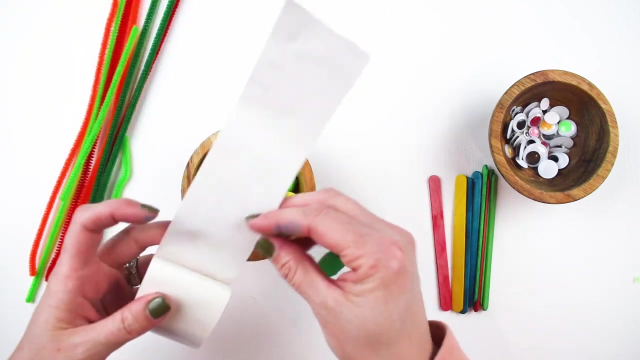 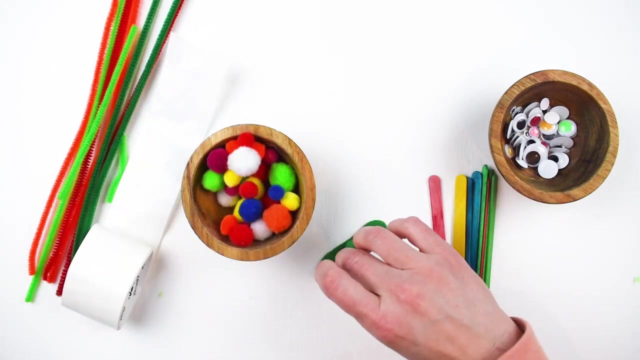 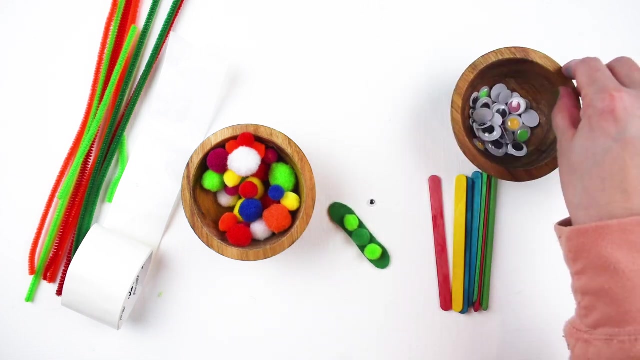 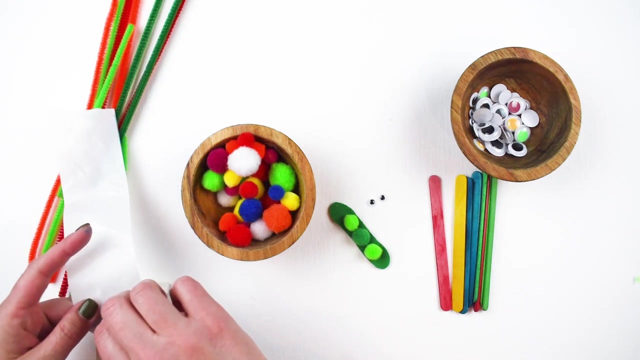 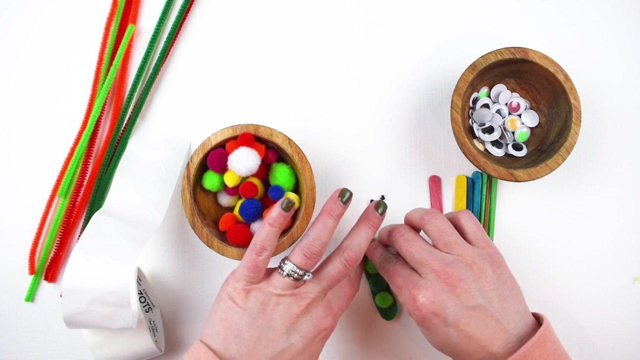 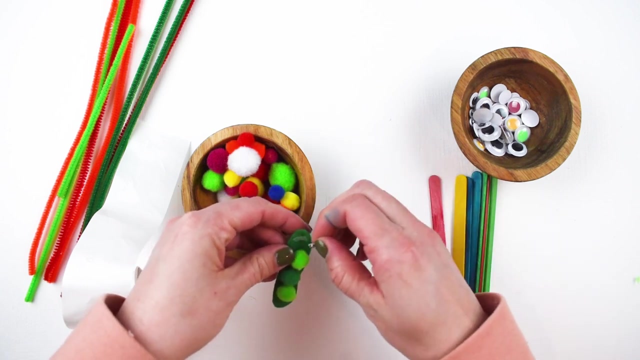 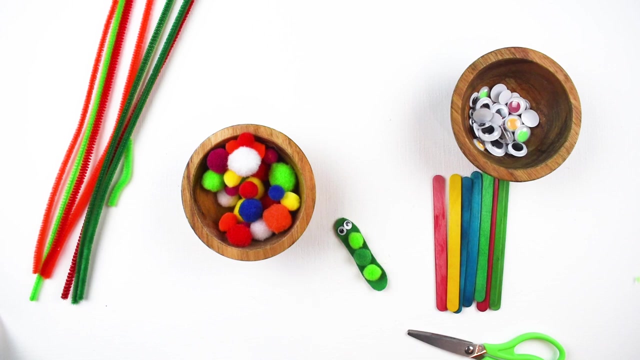 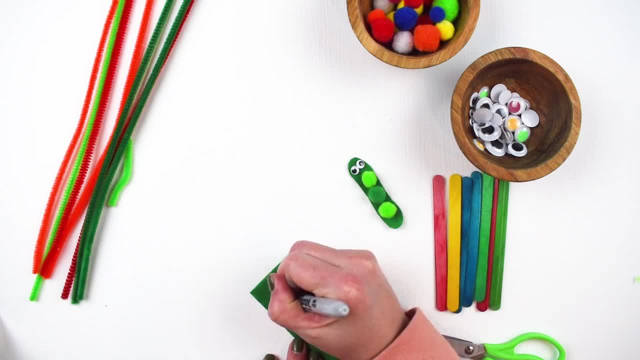 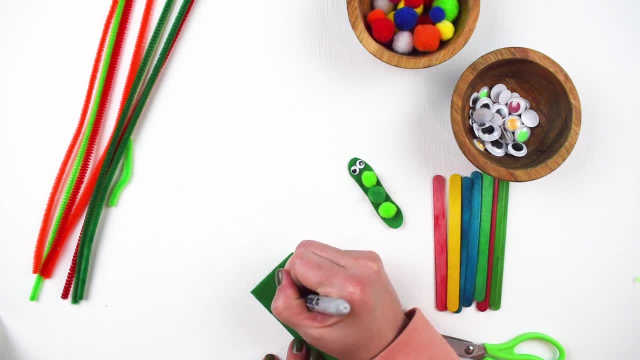 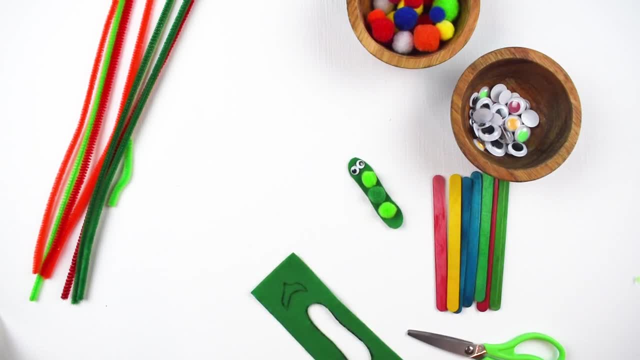 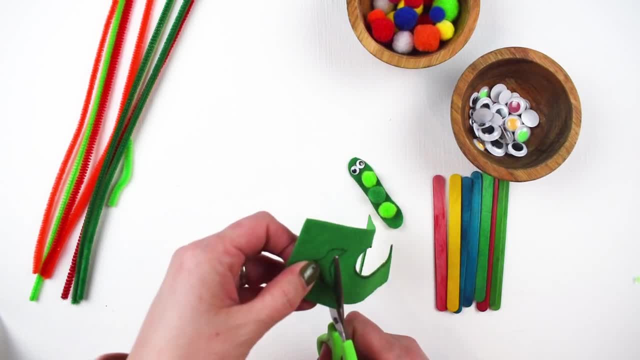 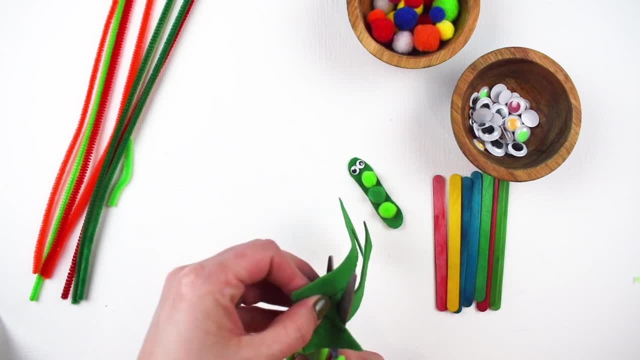 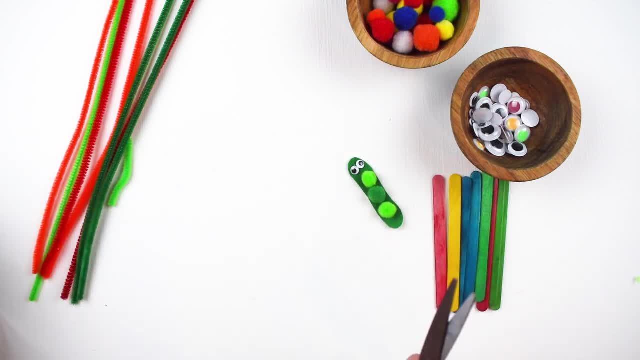 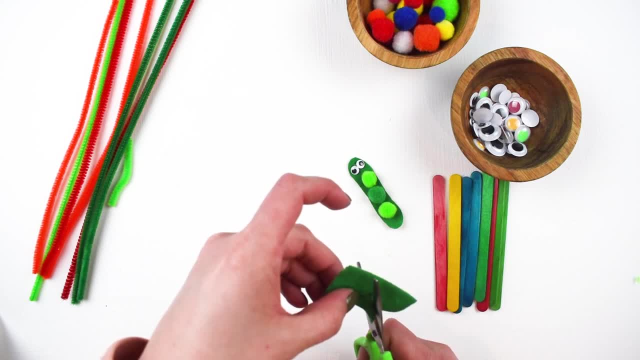 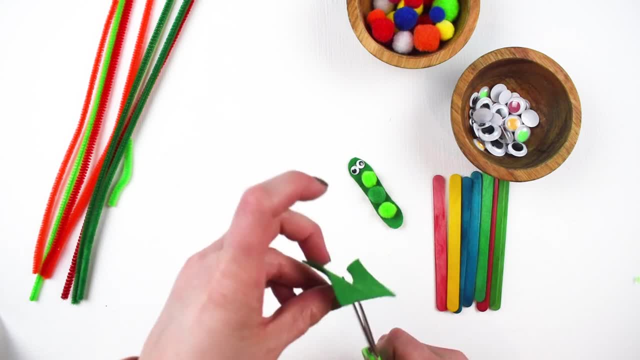 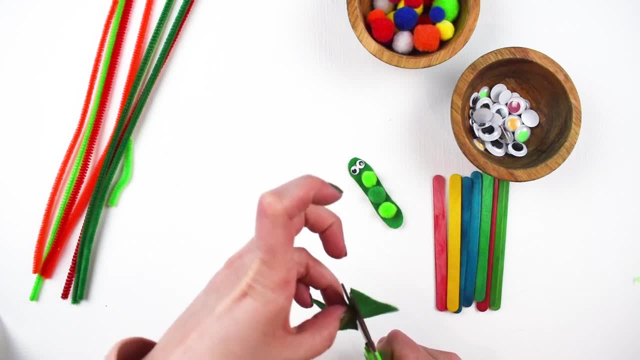 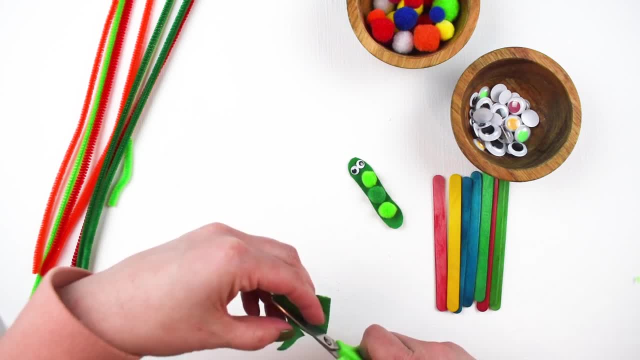